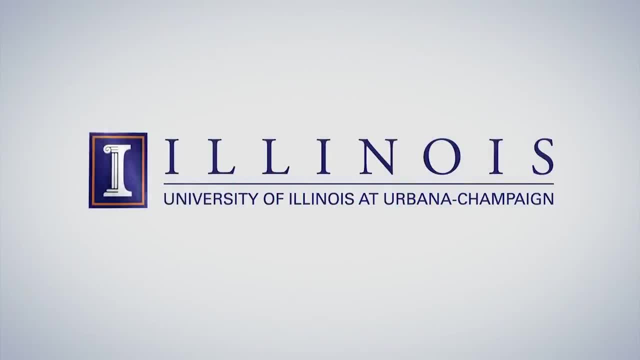 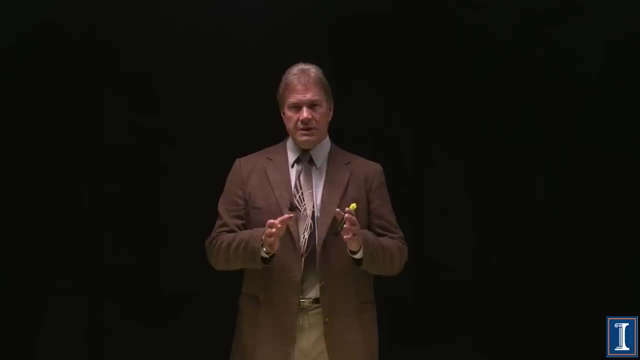 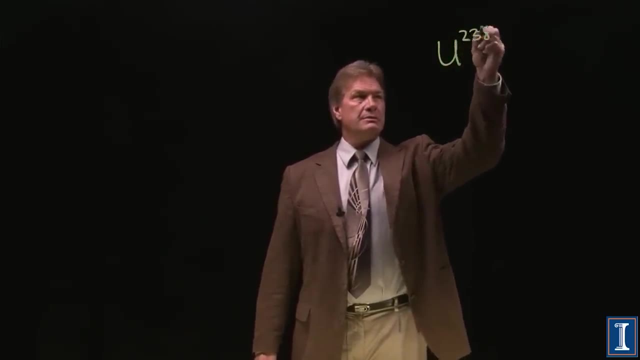 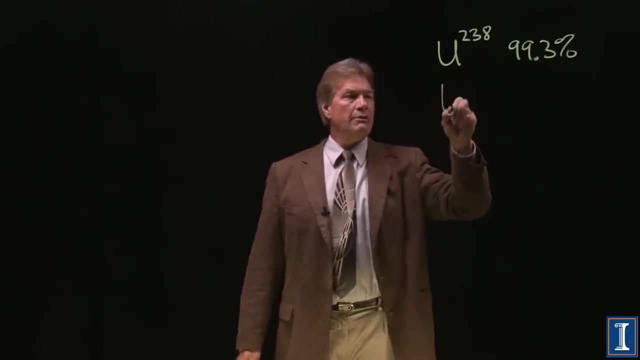 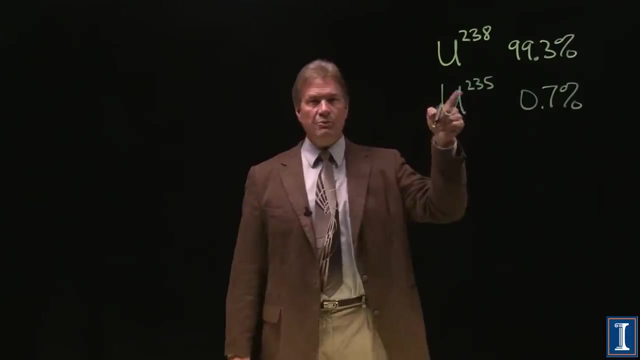 It turns out that uranium has two isotopes. Uranium 238 represents 99.3% of all uranium. Uranium 235 is only 0.7%, But it's this uranium 235 that is the useful thing for fission. 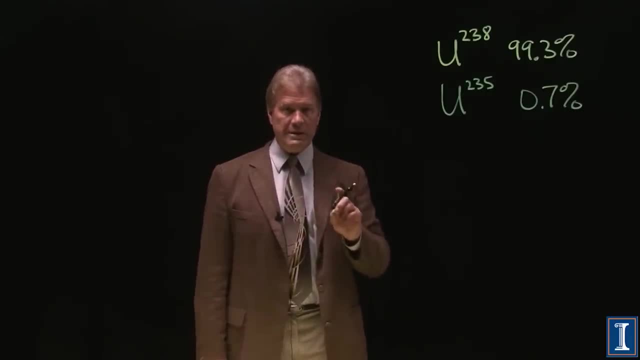 It's what we call fissile. Fissile means any speed of neutron can make it fission. Thermal neutrons, the ones you slow down with a moderator, make it fission at a very high rate. So this is what's useful as a fuel. 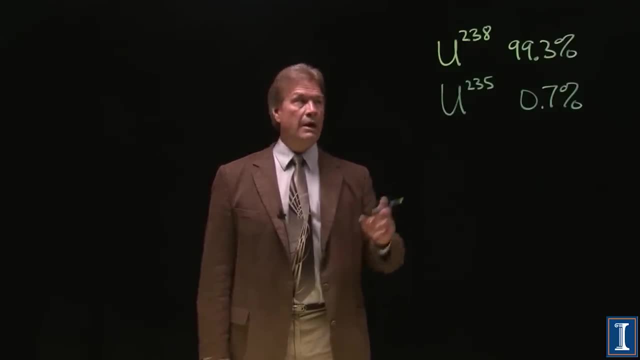 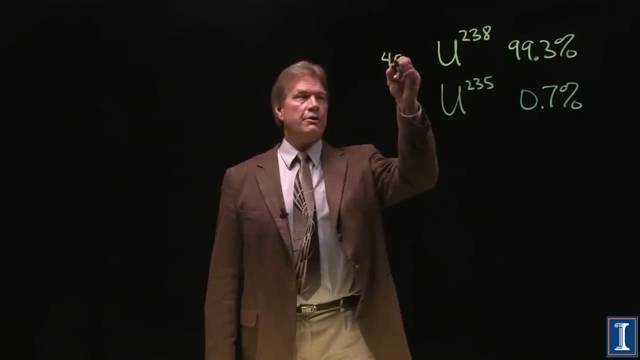 Or this is what's useful to make a nuclear bomb. Uranium 238 is pretty boring. It has a long half-life. The half-life of this is 4.5 billion years. Half-life of uranium 235 is only 0.7 billion years. 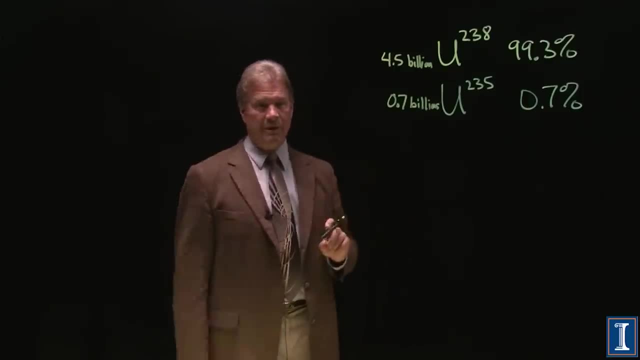 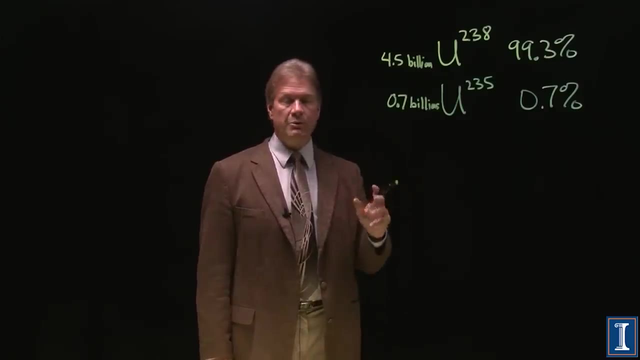 Compared to short half-life materials, these are fairly not radioactive because of their long half-lives, But it also means that the plentifulness of uranium 235 over history has clearly changed. But on our timescales of human activity, this is our ratio: 99.3% to 0.7%. 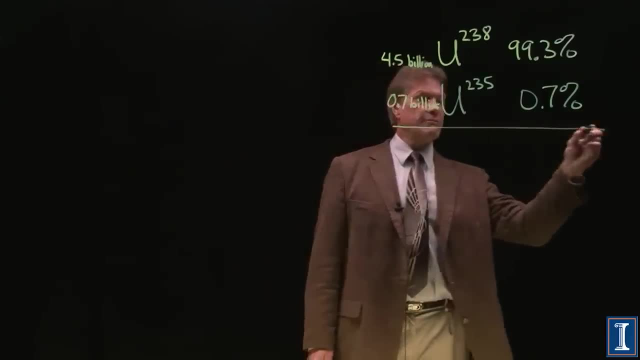 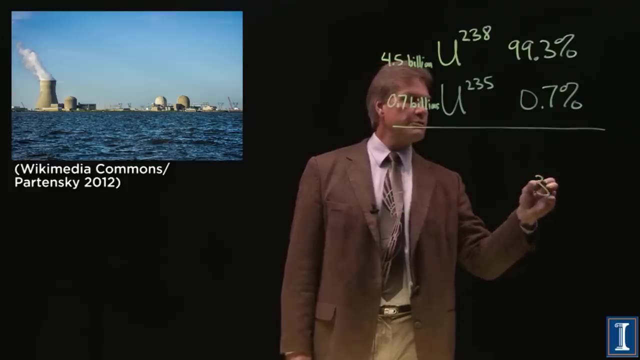 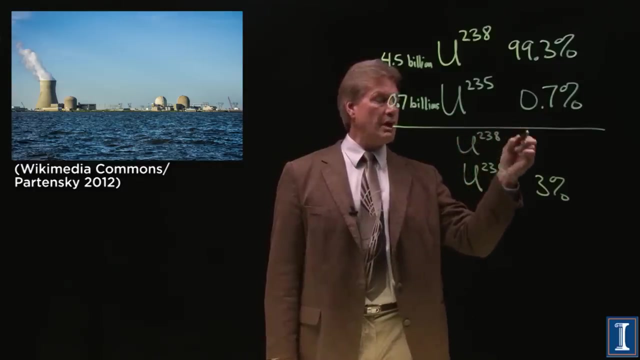 The thing is that this is how it occurs. naturally, If you want to run a reactor, you need 3% enriched uranium. That's a lot. That's a lot, That's a lot. That's really a lot. The outcarriage rate of uranium is what I want. 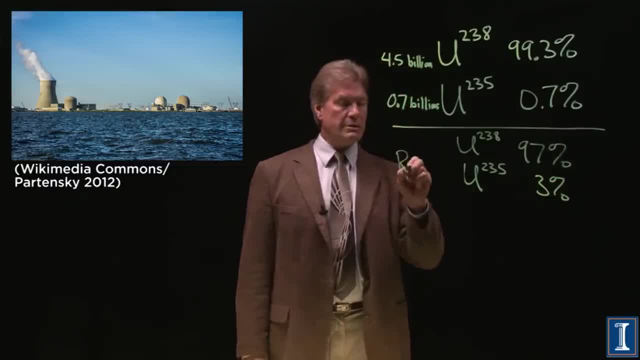 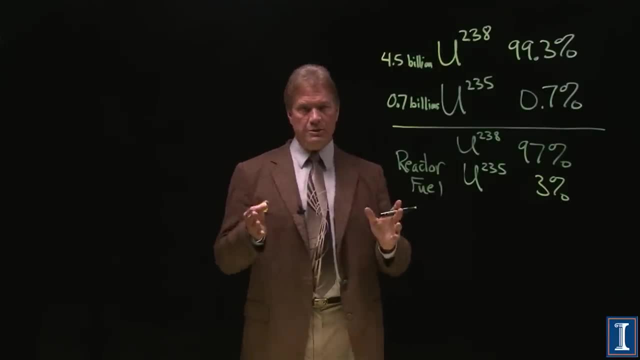 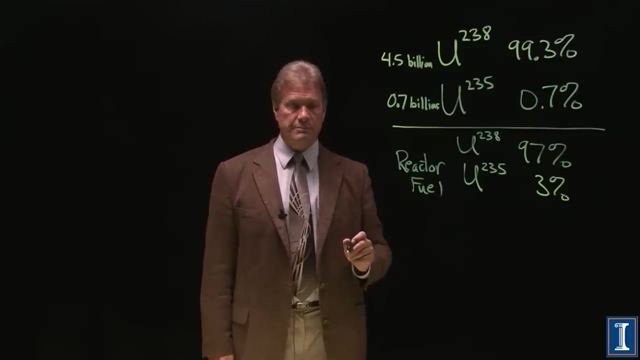 You get odors and highscenes, naturally, newリ a. The other issue is about the fuel. You may be wondering how cold theぜ. The process by which you get from a natural abundance to the reactor fuel is called enrichment, And I should mention that because it's in Wednesday's news. if you wanted to make a nuclear. bomb. it could be any time soon Where it's needed. Where it's needed, you actually have to get up to 90% uranium-235, which of course leaves the rest of it to 10% as uranium-238. The same enrichment scheme you use to take naturally occurring ore to reactor fuel. 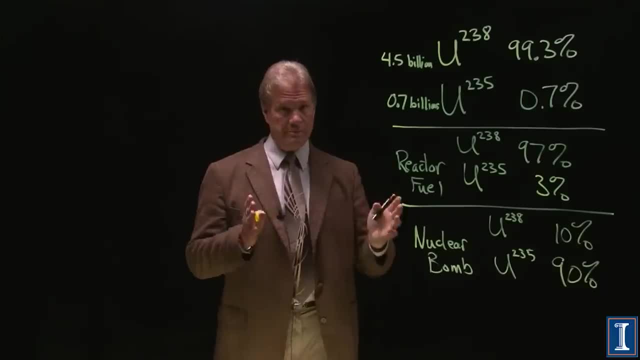 you could keep running for many, many more months or maybe years, and reach nuclear bomb-grade material. The thing about this is that uranium, as we've talked about, is a plentiful natural substance, So the key to making a bomb is being able to get it to this level of enrichment. 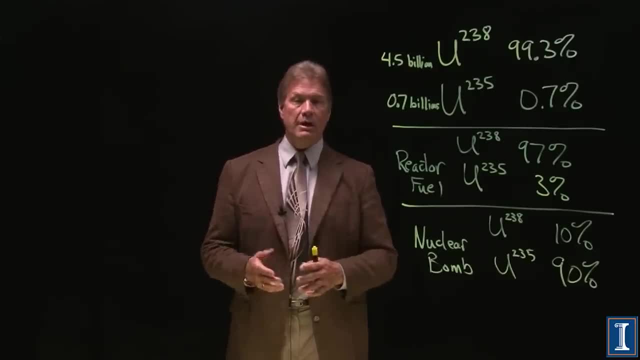 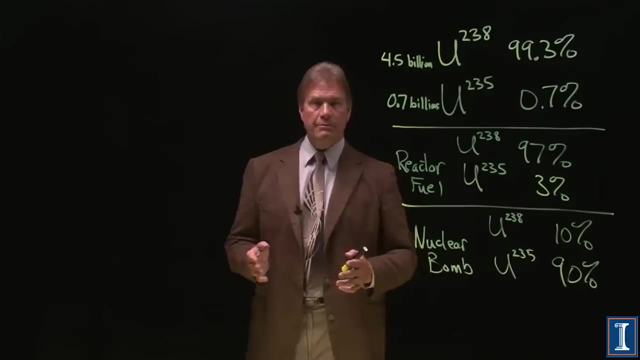 Once you have it, the knowledge of how to make a nuclear bomb is actually quite widespread. The gatekeeper to people, or really countries- having nuclear weapons is the ability to enrich it. So let's go back in time to where it was first discovered. 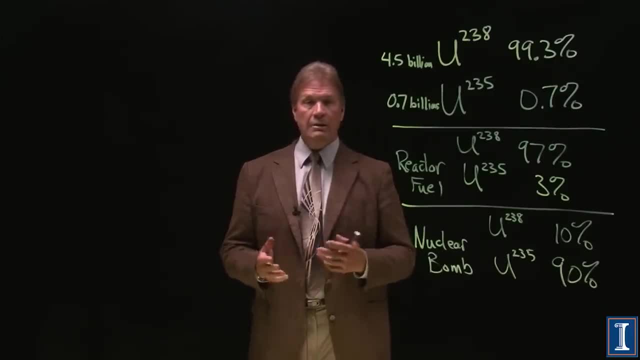 that you could make a nuclear chain reaction, and then, of course, that perhaps this could be something actually used in wartime, World War II. It was the genesis for creating the Oak Ridge National Laboratory. Enrichment is difficult because uranium-238 and 235 are the same chemical. Remember, every one of these uraniums has 92 protons- That's what makes it uranium- and 92 electrons. The difference is that the 238 has 146 neutrons versus 143 neutrons for the uranium-235.. The only difference is this: less than 1% mass difference. 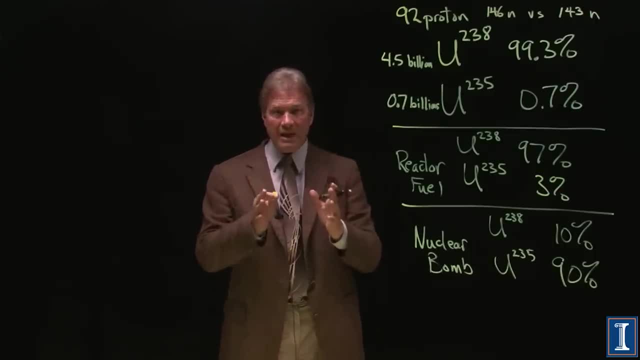 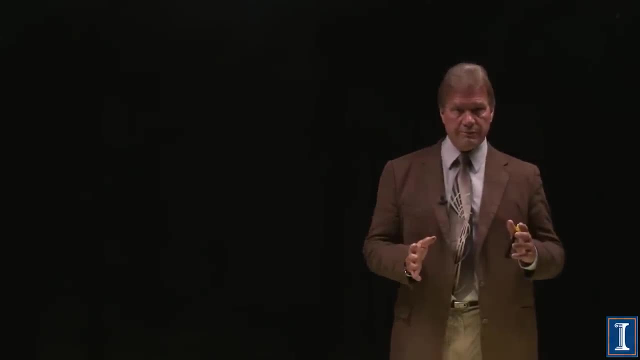 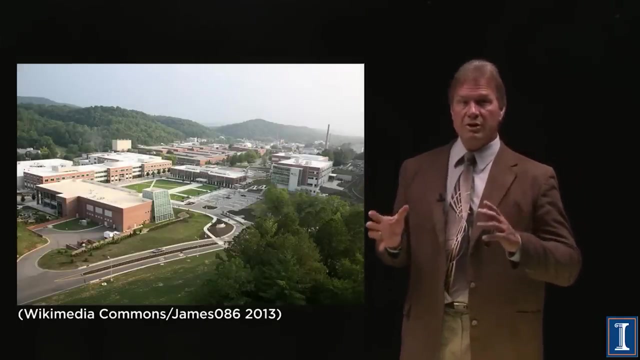 And we somehow have to utilize that mass difference to be able to enrich it. Enrichment is a huge effort, In fact. in the 1940s the US created in part Oak Ridge National Lab for this very purpose. Now this is a modern picture, but still the National Lab was nestled. 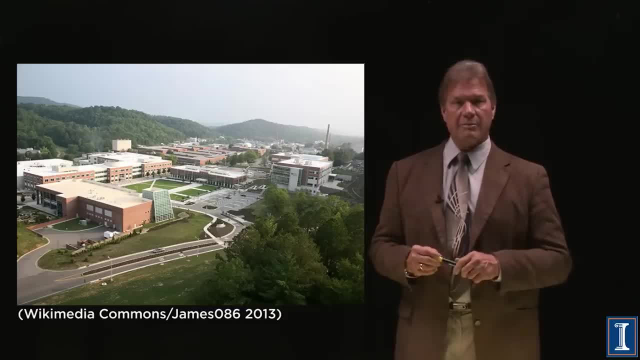 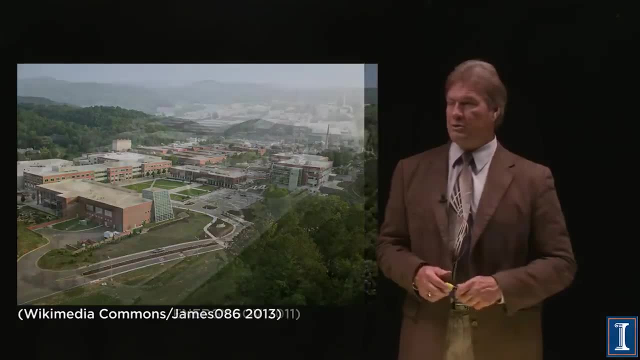 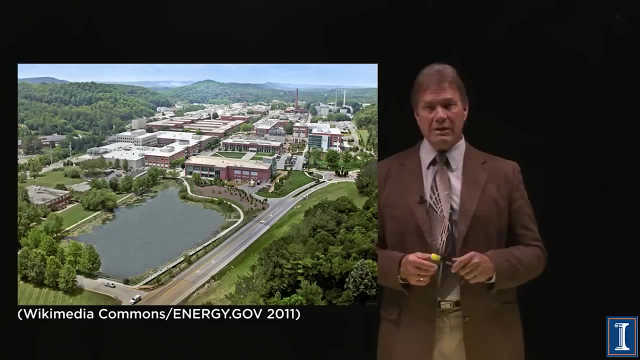 in the middle of the Tennessee mountains, about an hour away from Knoxville, Being a place where they could enrich uranium. There's another aerial picture of the lab showing you. it's kind of deserted around there. It's also in some beautiful hilly area and a convenient power feed away. 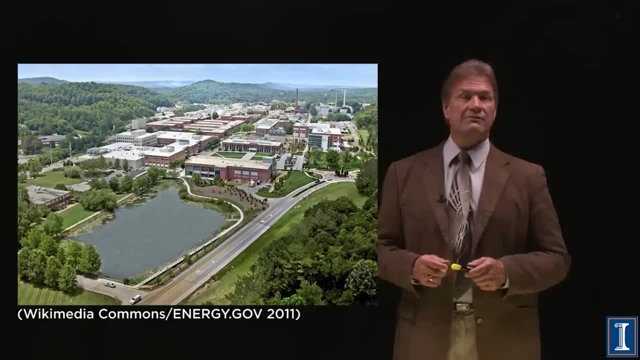 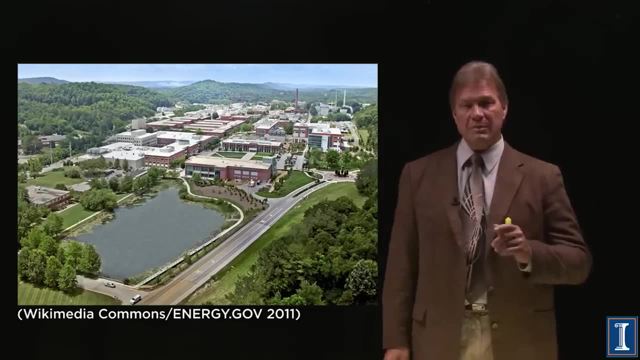 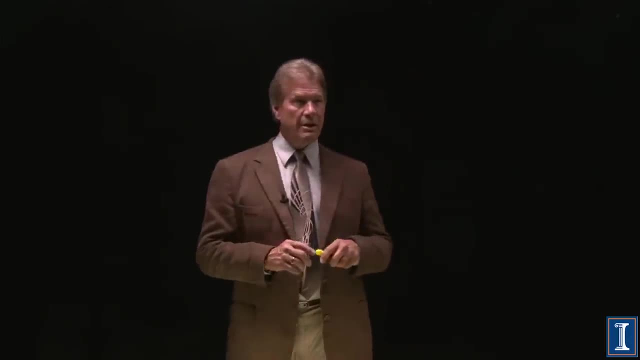 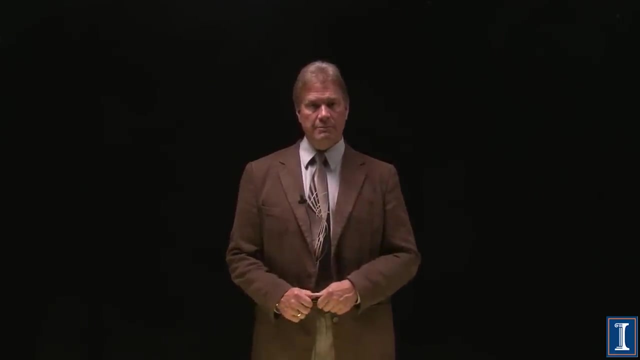 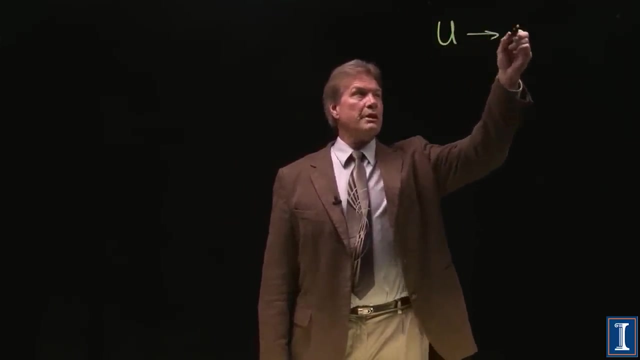 This is what we have. The idea to use this giant plant was somehow to utilize the mass difference between the two isotopes of uranium. First, to do that, you have to turn it into a gas, So the uranium fuel was made into the gaseous uranium hexafluoride. 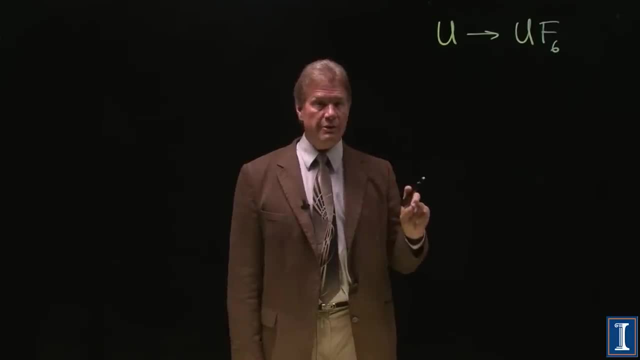 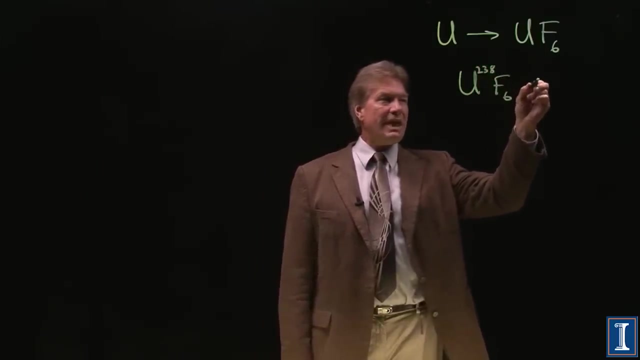 And this dilutes the mass difference even further, because you've got the fluorine molecules right. So now our mass difference is even greater. So now our mass difference is exceptionally tiny. But U238F6 is slightly heavier than uranium-235F6, very slightly. 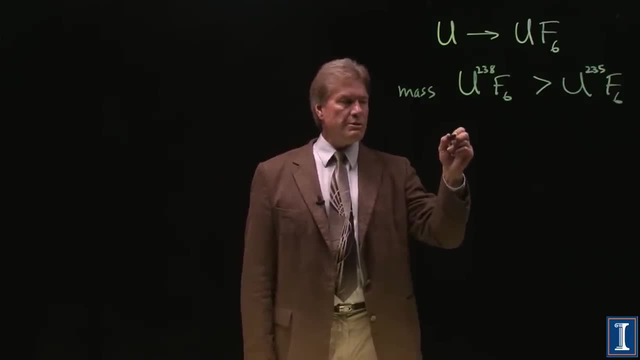 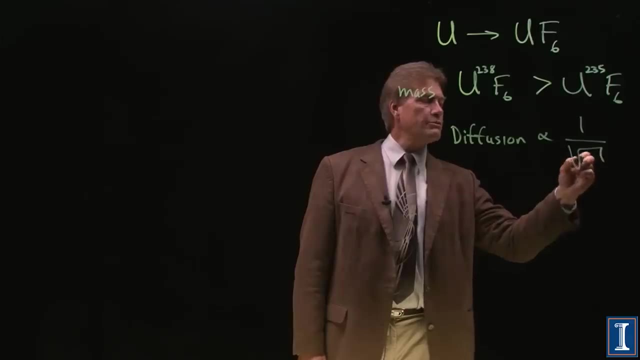 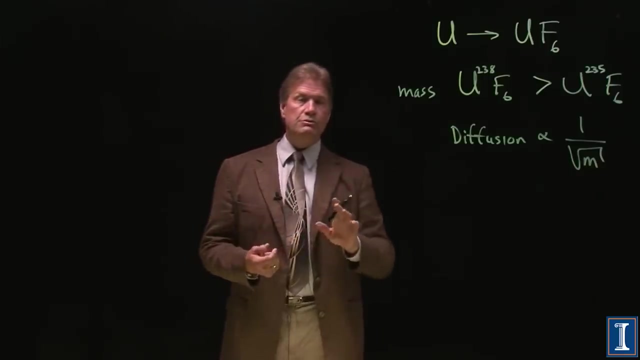 If I use diffusion, diffusion happens proportional to 1 over the square root of U238F6.. If I use diffusion, diffusion happens proportional to 1 over the square root of U238F6.. of the mass. So a lighter substance will diffuse slightly faster than a heavy substance. 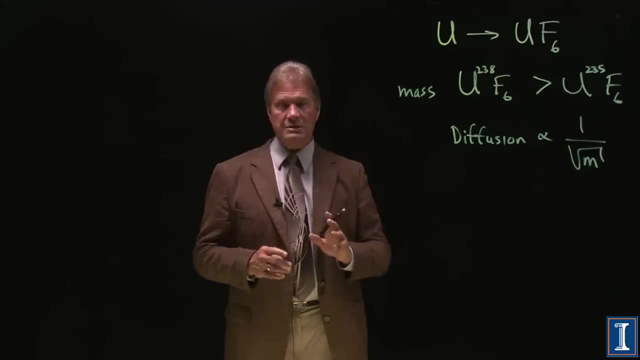 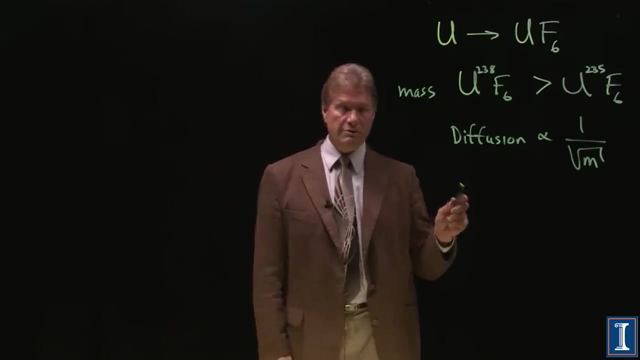 This was the thought of the gaseous separation plant at Oak Ridge. Basically, take a filter and put something through it And the heavier stuff won't go through quite as fast. So you need to build a lot of machines because the separation factor using gaseous diffusion 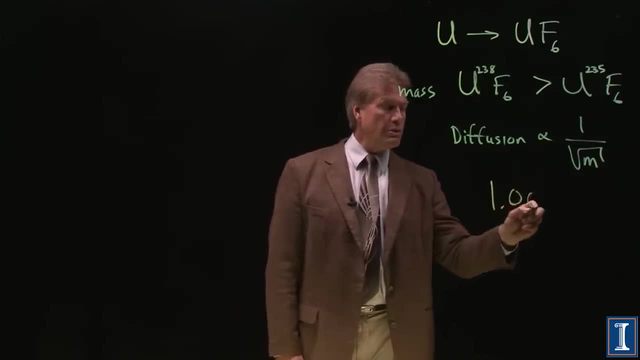 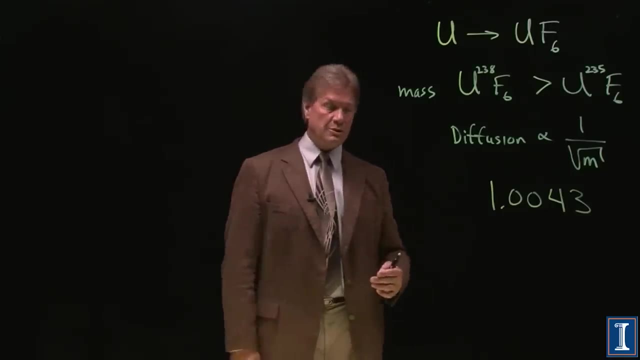 between the two different masses is only 1.0043, four thousandth of 1% increase in separation, And after all we're trying to get from 0.7% if we're making a bomb all the way to 90%. 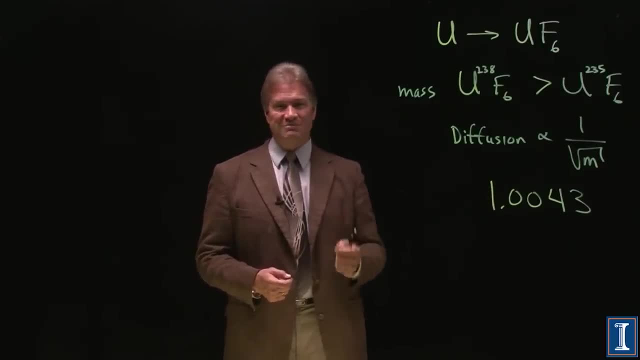 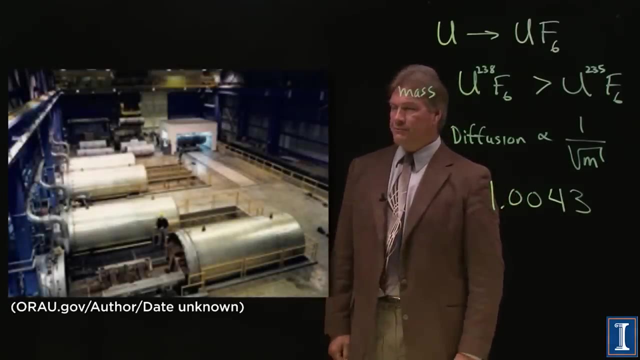 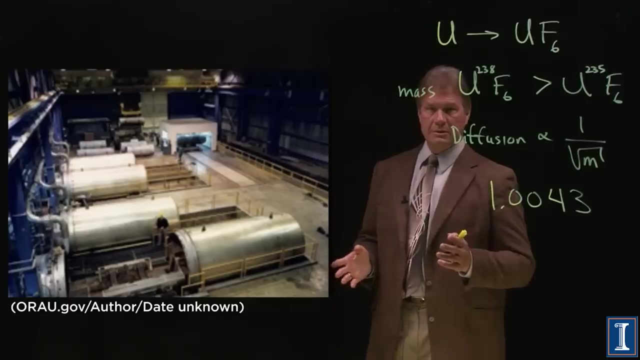 and every stage only improves you by this much. Here's a picture of a gaseous diffusion system at Oak Ridge. These are large, large containers. and there aren't just four of them, there are thousands. Let's look at a diagram to see how this works. 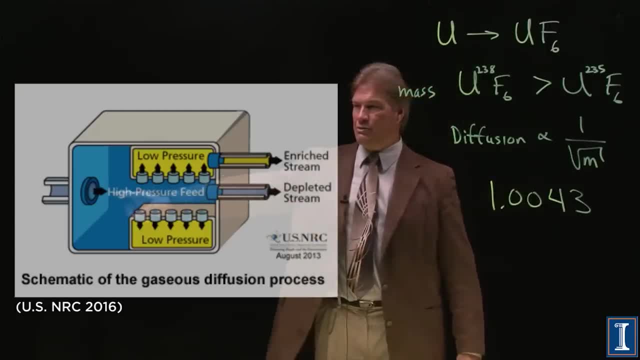 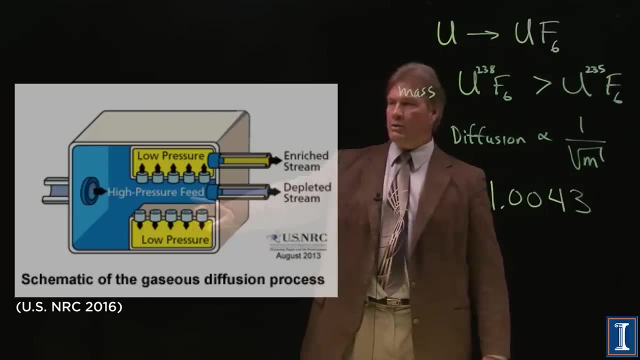 So the high pressure gas, the UF6, comes in, And these are all your little coffins, These are your coffee filters, your diffusion membranes And, of course, what's going to diffuse faster, Something that's slightly less massive, the U235.. 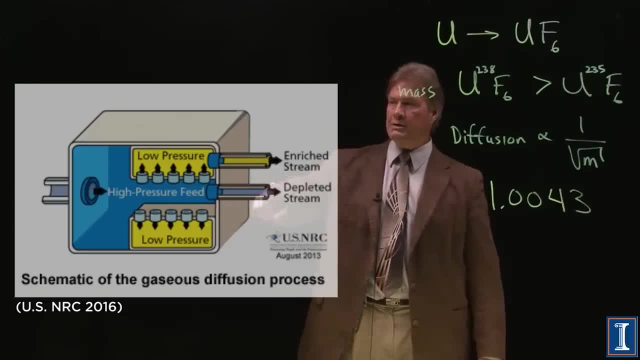 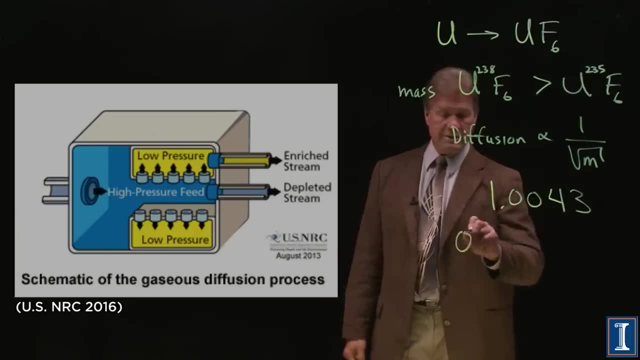 So here would be the enriched stream and here would be the depleted stream. Not by some huge factor. remember this? 1.0443?? That means, if it starts at 0.7, right, the depletion and the enrichment fraction goes to something like: 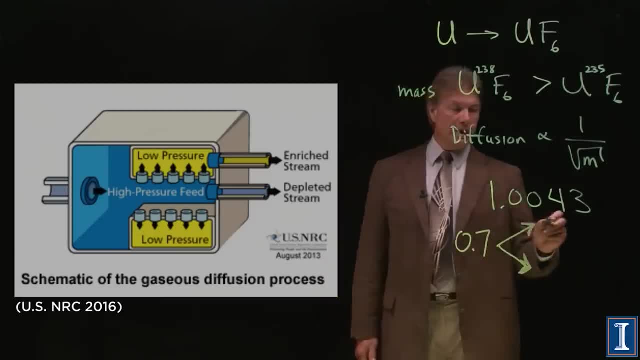 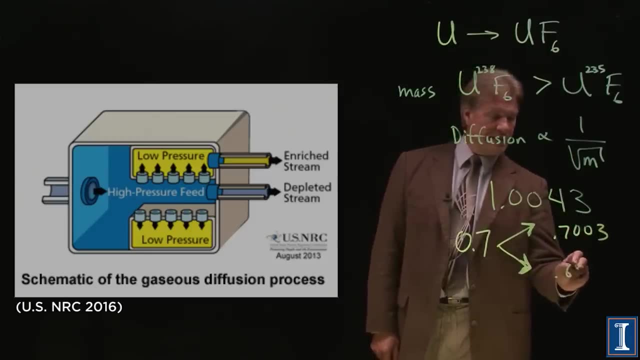 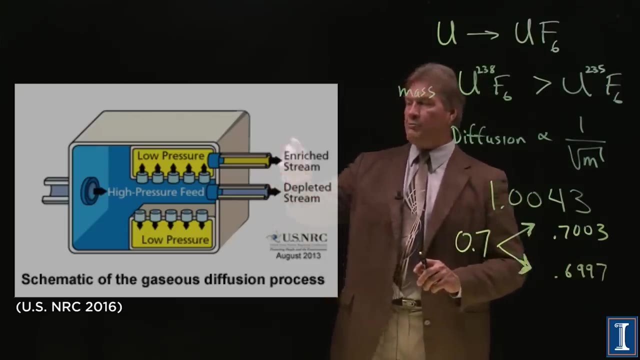 Well, multiply that times 0.7.. We've got something like 0.7003 and 0.6997 through one stage. Then you would take this enriched stuff, put it through another system like this and it would go up a little bit further and a little down further. 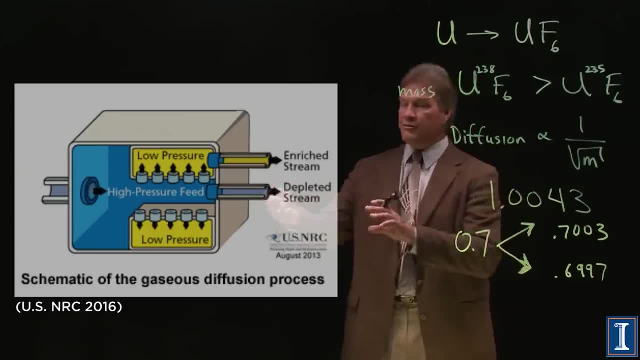 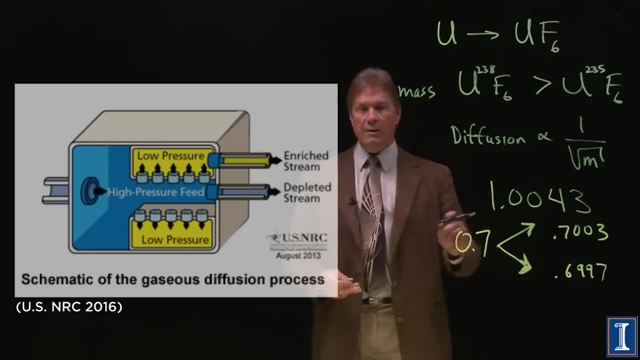 You have to take the stuff that was de-enriched and put it back into the first one And eventually, through massive numbers of these, These machines, Years of doing this, you could get up to the desired enrichment. This was 1940s technology. 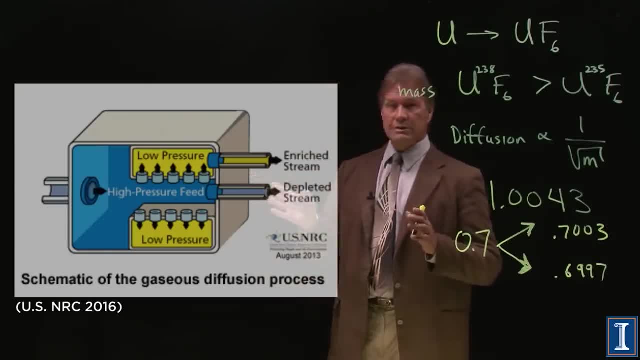 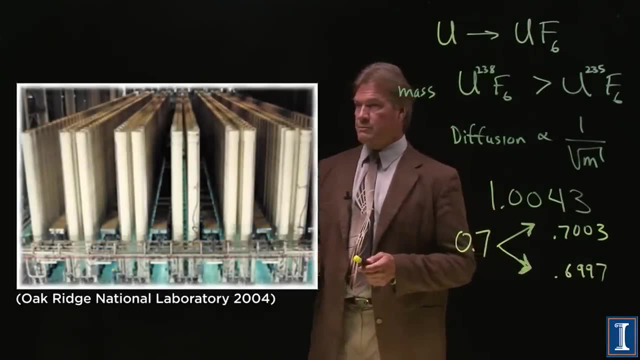 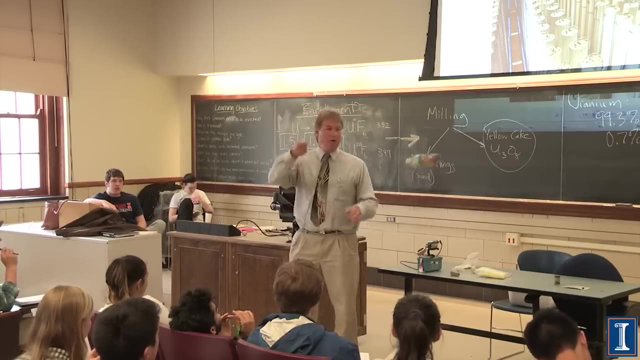 What about today? Today we go to something much better called a gaseous centrifuge. Here are pictures of centrifuges And, as you might imagine, and how this demo shows, if you spin something, the heavier part goes out to the side. 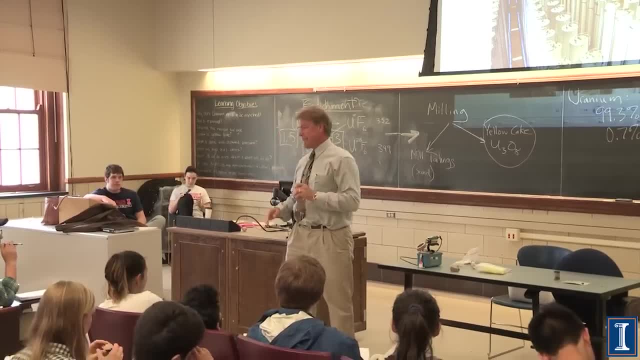 Let me hit it k k into zero. squared: heavier part goes out to the side, the lighter part stays in the middle. these: 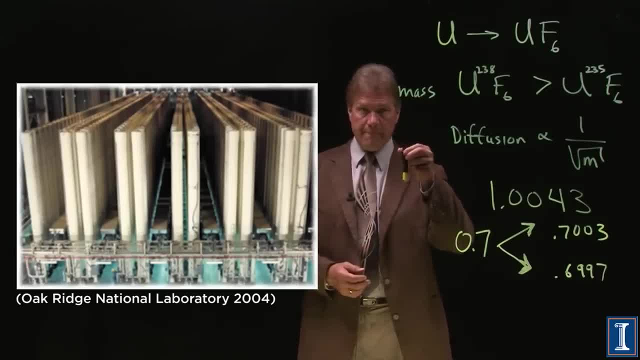 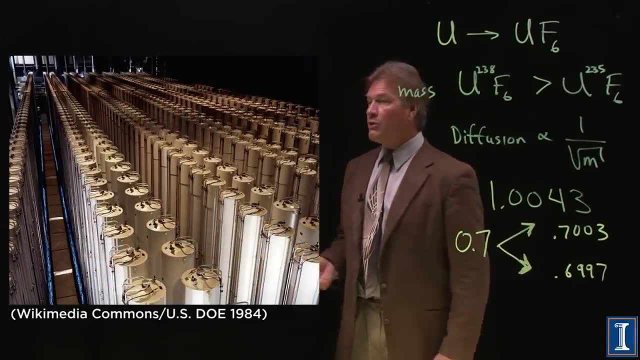 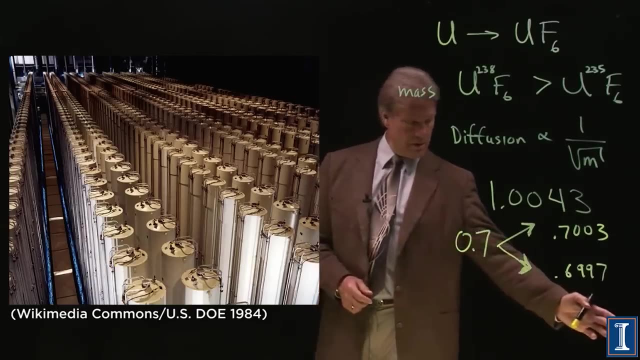 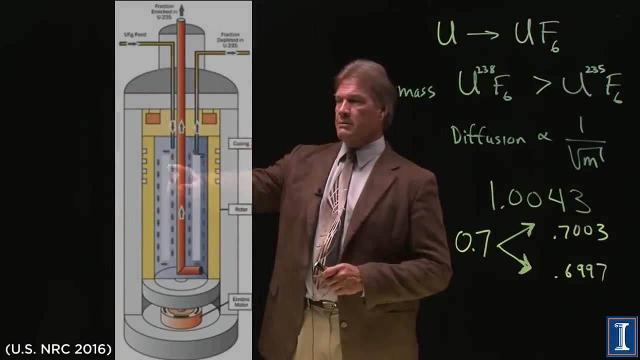 centrifuges spin like tops- here's another picture- and you need many of them, of course, but their volume is nowhere near as massive as the volume of the types of gaseous diffusion. a diagram that shows how they work is again a very similar principle: that you feed the gas in and that, as this spins in a circle. 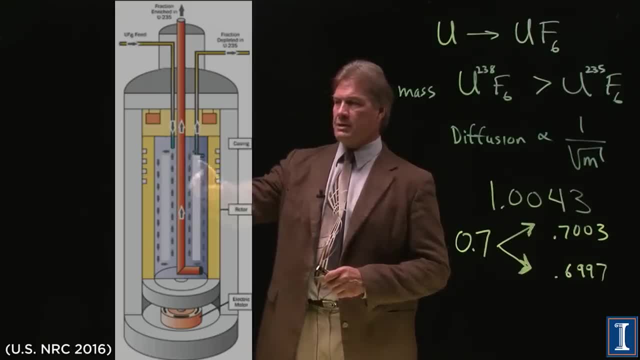 the heavier substance comes to the outside of the cylinder, that would be the u-238, the depleted uranium, and from the center of the column you get the lighter gas, that is the enriched u-235. the separation factor for a gaseous centrifuge can be as high as the center of the cylinder and the center of the. 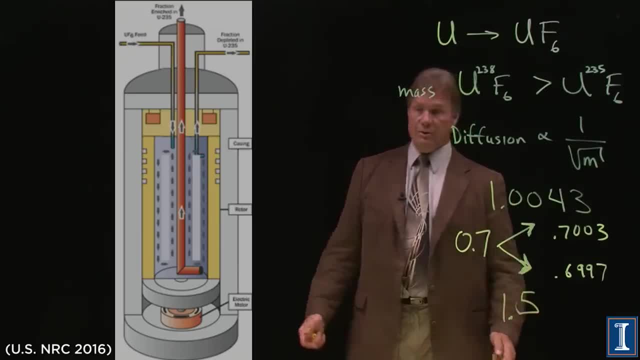 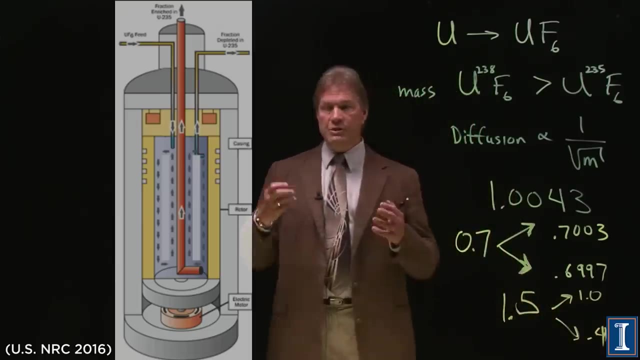 cylinder can be as high as 1.5. that's great. you go from 0.7 to all the way up to something that's like 1 right and down to something like 0.4 or so, all in one step. many fewer steps are needed to be able to get up to the enrichment. 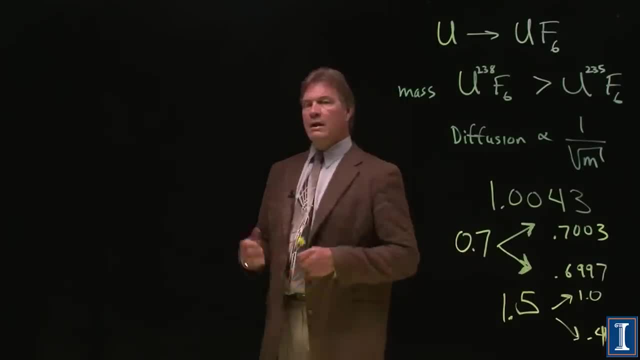 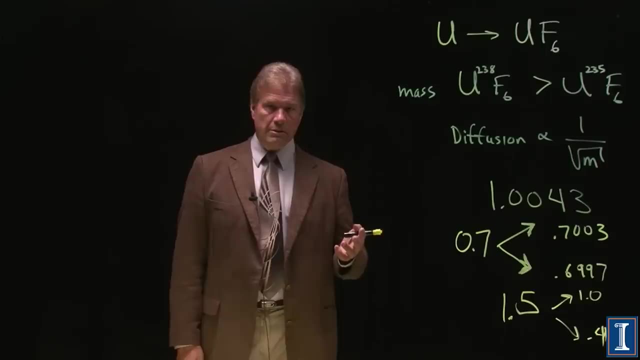 level that you would like. that also brings us to a very timely subject, and that's the subject of the next slide: Iran. Iran has centrifuges to enrich fuel. according to Iran, they want to have a domestic nuclear power program and they need to make their 3% level reactor. 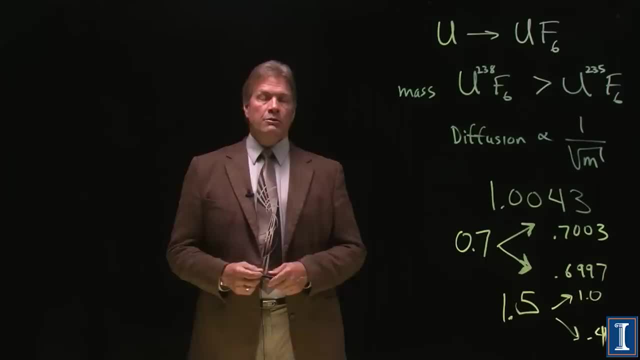 fuel great. the worry of the West is that they will continue running the centrifuges and they will get up to the 90% level needed to make a nuclear bomb. they say no, of course we're not going to do that. the West says okay, well, let us. 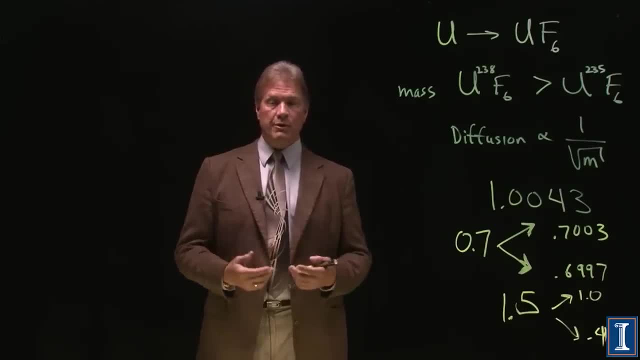 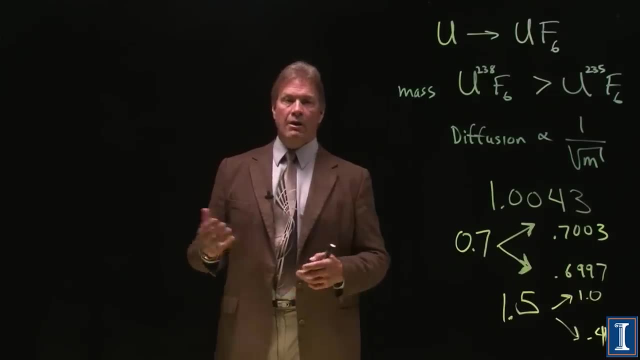 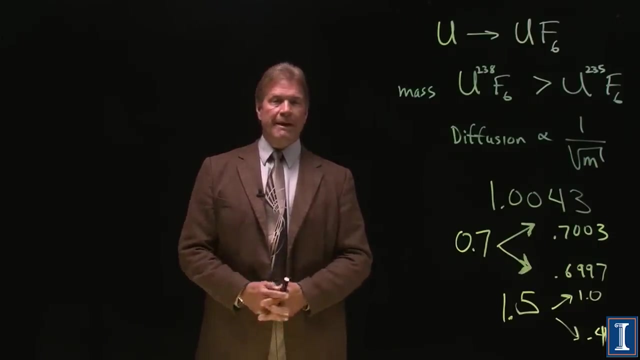 inspect and even if there's an agreement, there's a worry that is there some diffusion plant one doesn't know about? is there some centrifuges you don't know about? are they really being truthful? have they really already perhaps made the 90% enrichment material? I'm not a political scientist. I'm not teaching you. 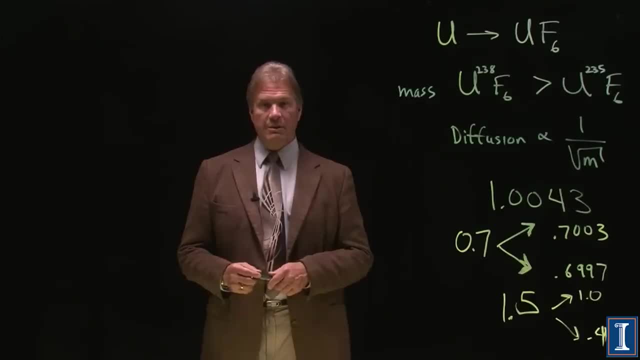 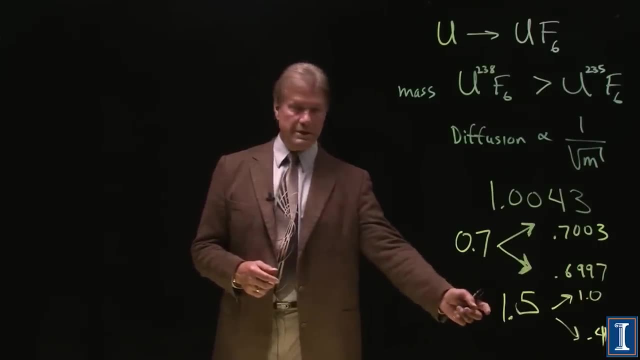 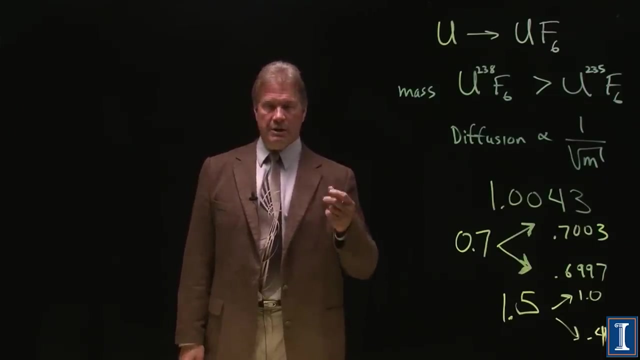 of course, on politics, I don't know what the answers are, but I want you to understand technical things that are involved. making a gas centrifuge that can get this type of separation factor is not trivial at all. it's extremely high precision device that needs to run extremely tight tolerances. but if you